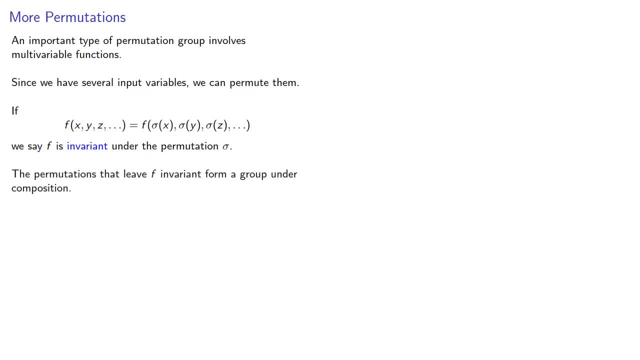 that leave f invariant form, a group under composition. For example, let's find the group of permutations on the variables, under which f of x, y, z equals- x squared plus y squared plus z squared- is invariant. Now the function is the sum of the squares of the input variables. 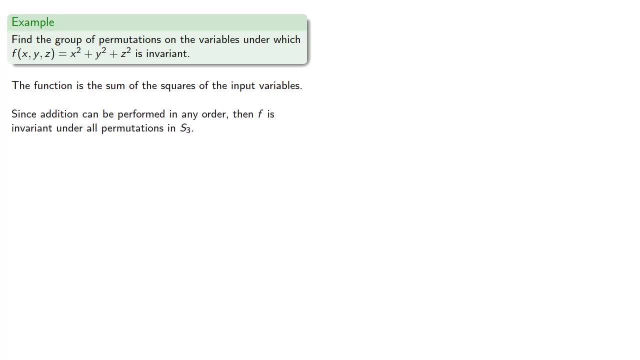 Since addition can be performed in any order, then f is invariant. f is invariant under all permutations in S3.. What about a function like f of x, y, z w equals x y plus z w. So let's begin by considering what happens if we map x to a later variable, Since our 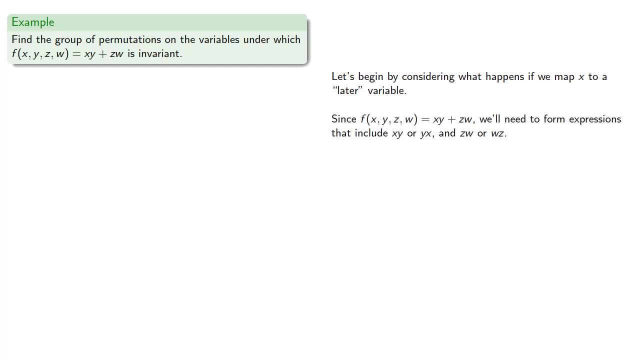 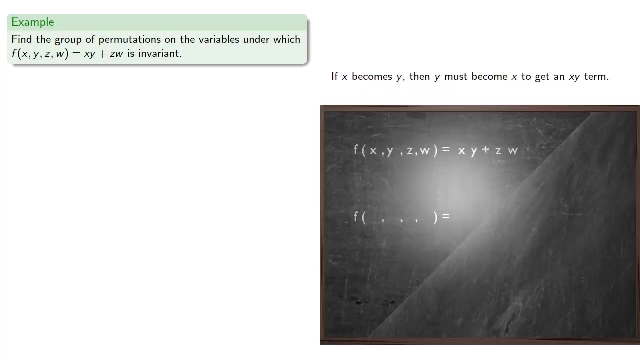 function is a product of x and y. with a product of z and w, we'll need to form expressions that include x, y or y, x, and z, w or w, z. So if x becomes y, then y must become x in order to get an x- y term. 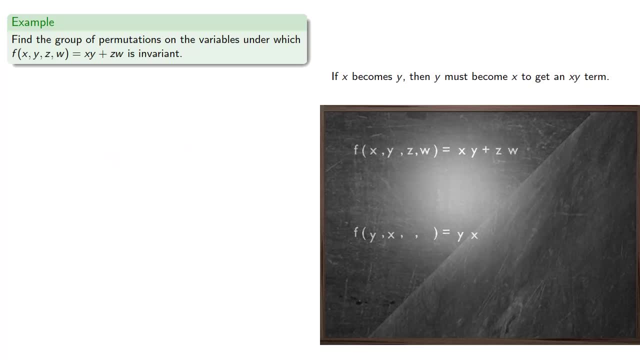 Meanwhile, the variables z and w. we could leave them alone, And that gives us this permutation. Or we can switch z and w, and that gives us this permutation. Or if x becomes z, then y must become w, because we need to get that product- z, w. 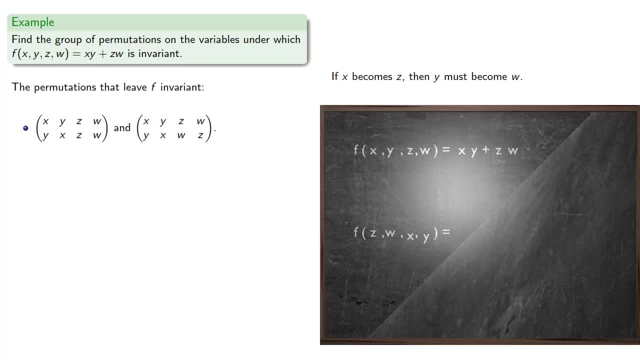 And again, z could become x and w could become y, Or z could become y and w could become x, Or maybe x could become w Again. in order to get this z w product, that means y has to become z. and our last: 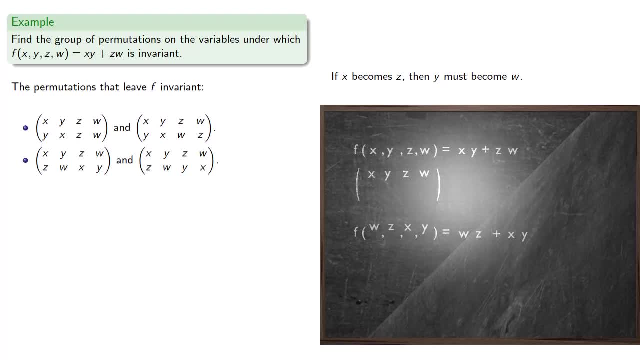 two variables can either become x and y, Or they could become y and x. Now let's consider anything that permutes y. If y becomes any later variable, x will also have to change, and we've already found all those possibilities, so we don't have to worry about permutations that change y and a later. 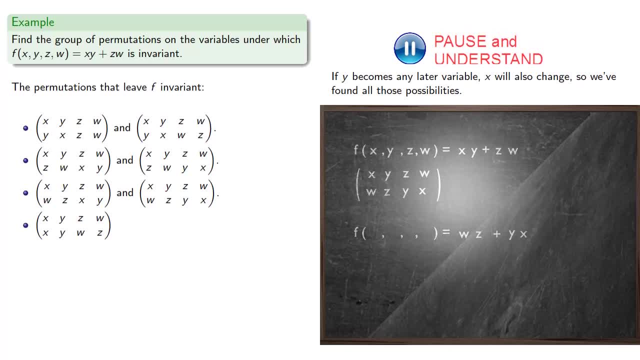 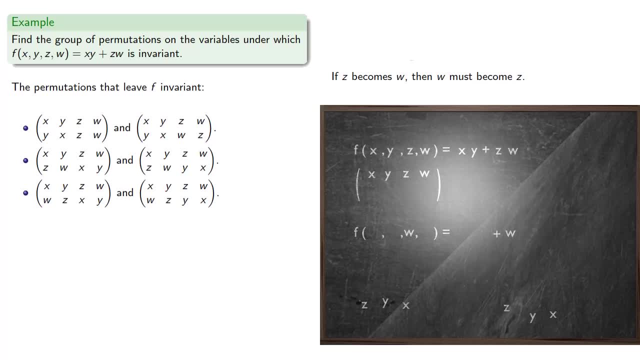 If z becomes w, then w must become z, And we'll leave x and y alone, because we've already considered all permutations that move x. And, let's not forget, we also have the identity permutation e, And so all together, there are these permutations that leave f invariant. 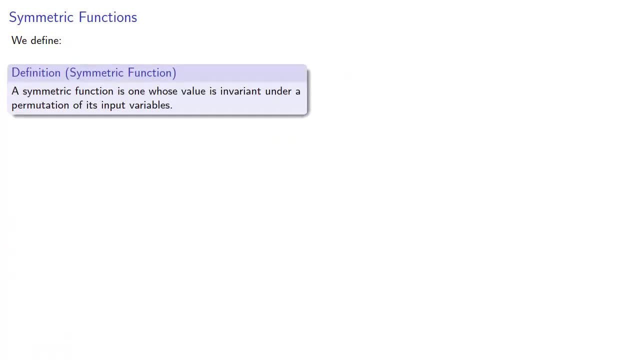 We define f as a product of x. We define a symmetric function to be one whose value is invariant under a permutation of its input variables. Now, if a function isn't symmetric, that means some permutations will yield different values. Let's take a look at that. 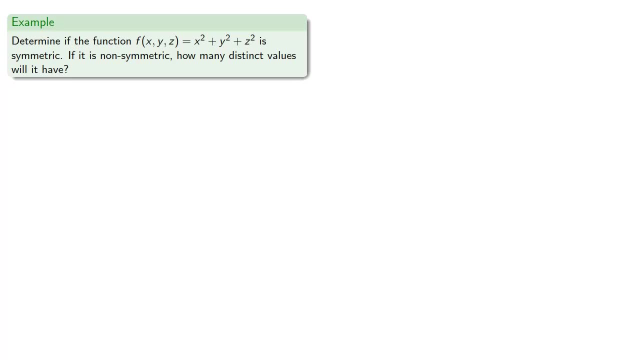 So let's determine if our function is symmetric, and if it's non-symmetric, how many distinct values will it have? Well, we've already determined that this function is invariant under all permutations, and so there's only one permutation, There's only one function value, namely x squared plus y squared plus z squared. 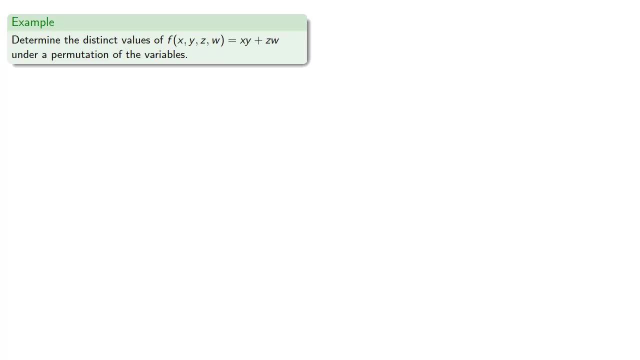 On the other hand, consider something like xy plus zw. We already found the group of permutations under which f is invariant and it's not all permutations. so there are distinct function values. So the distinct values will be the function as defined, because there is a group of permutations. 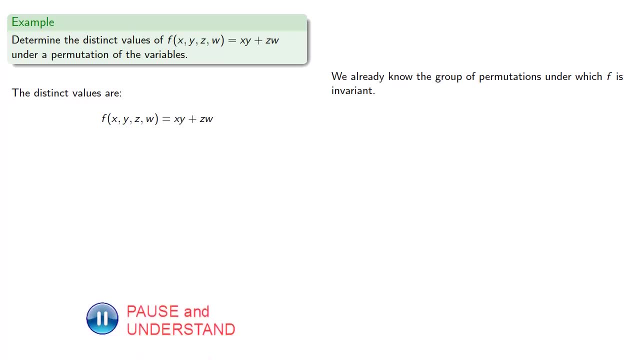 that produce the same value. Now, to produce a new function, value x has to be multiplied by either z or w, and this leaves only two other possibilities: f of xz yw, that's xz plus yw, and f of xwyz, that's xw plus yz. 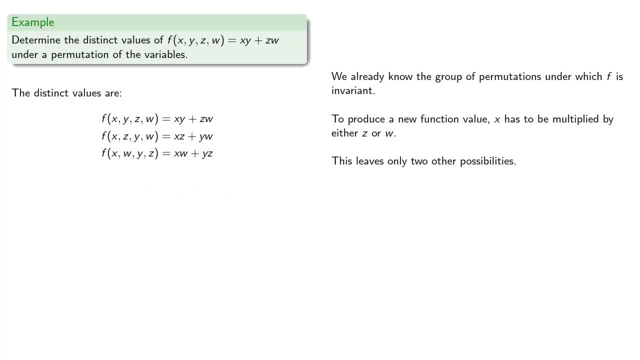 And so let's think about this: There is a group of permutations that give us this value, xy plus zw, and then every other permutation is going to give us one of these other two values. And this turns out to be very important, and we'll take a look at that in a little while. 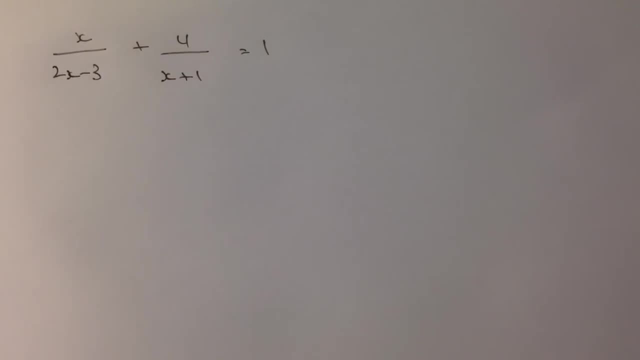 Hi, in this particular video we're going to be looking at solving these values of x, So this is a little bit tricky now that we've been given this particular question. It's a bit like when we deal with adding two fractions together. So, just as an example, let's say we looked at something like a quarter plus a third. 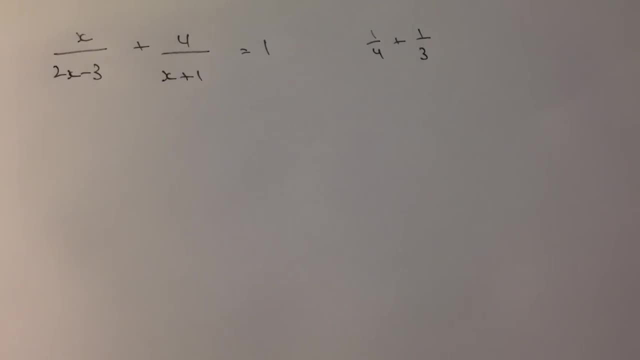 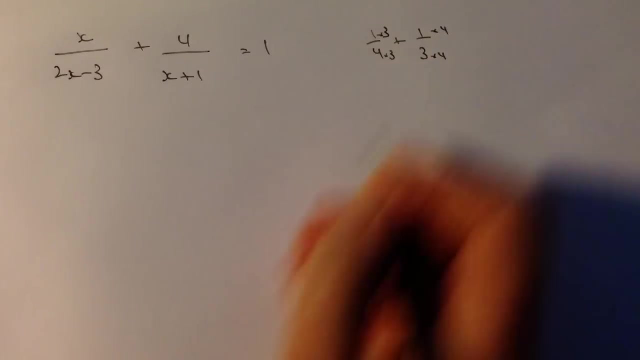 What actually happens with a quarter plus a third? Well, actually, what we do is we create the lowest common denominator, which, in this particular case, would happen to be 12.. Practically, what we do is we multiply this by 3 and this by 3 and this by 4 and this by 4.. 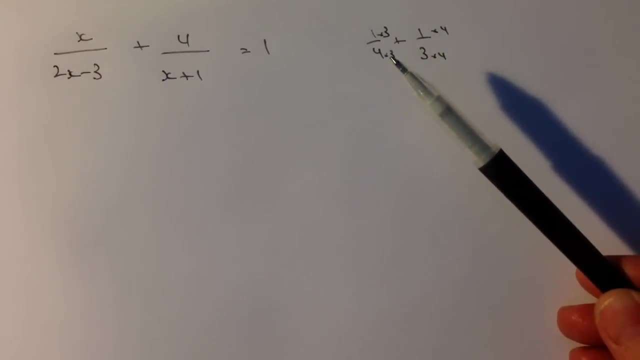 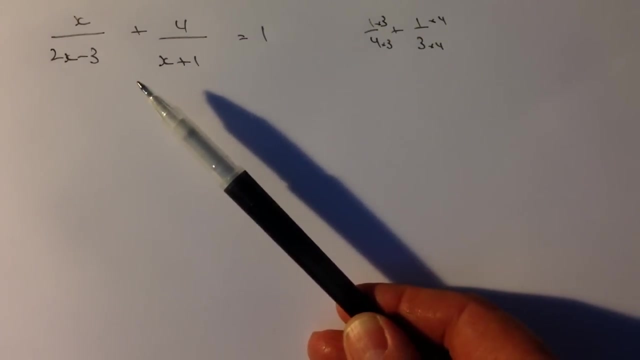 So what we're doing is we're taking these two bottom numbers, these two denominators, and multiplying the two together and creating a multiple. Now, in this particular case, it is the lowest common multiple, And we're going to do exactly the same with this particular question. 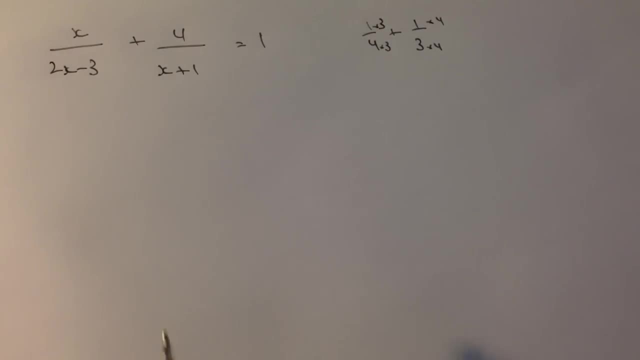 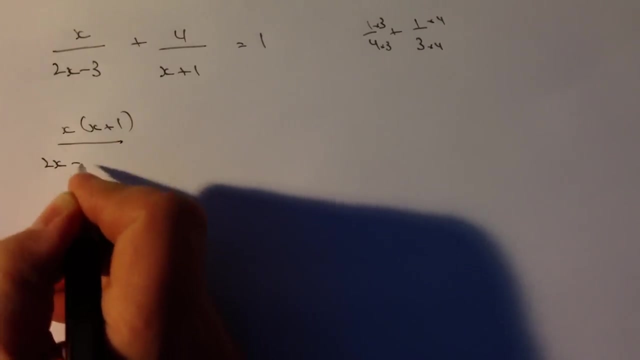 So what we're going to do there is: we're going to say that we're going to take this fraction and we're going to multiply this fraction through by x plus 1.. So what we end up with is x times x plus 1 over 2x minus 3 times x plus 1.. 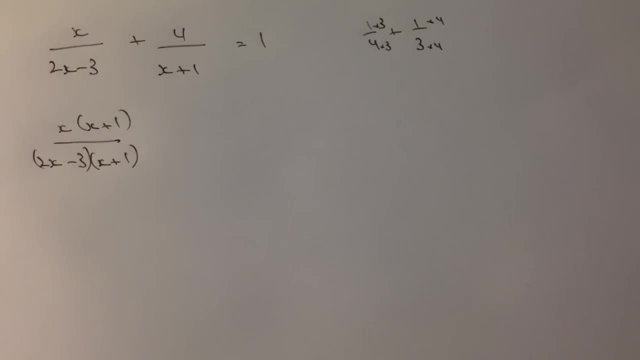 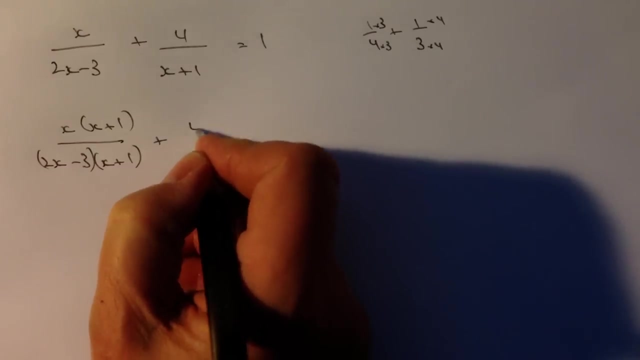 And we put it into brackets like that just to make it a little bit tidier. So that did work. So that deals with the first fraction. The second fraction, we do exactly the same. So this time, however, I'm going to multiply by 2x minus 3..